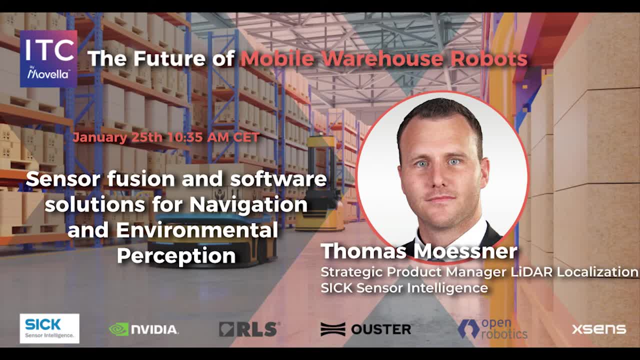 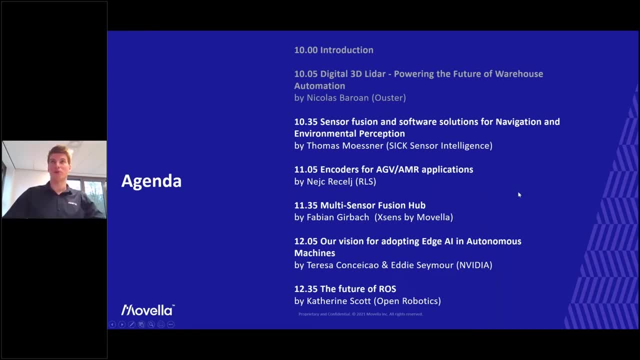 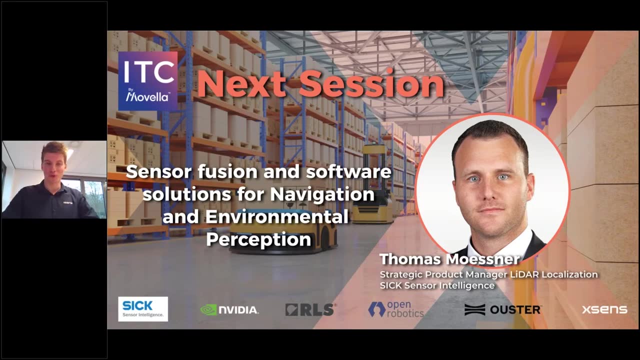 Next session is Thomas from SICK, and actually I want to go to the next slide where we see- and I want to hand the word over to Thomas: Thomas, if you could unmute yourself, put on your camera and share your screen, then the floor is yours. 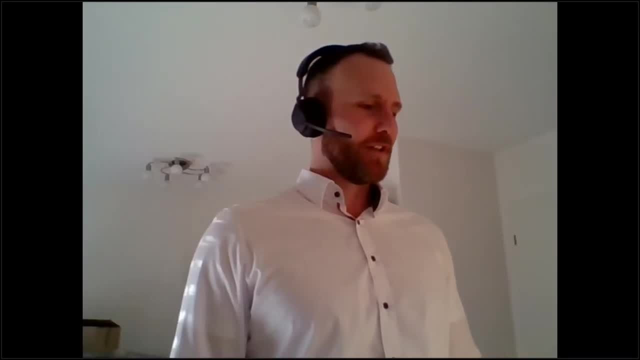 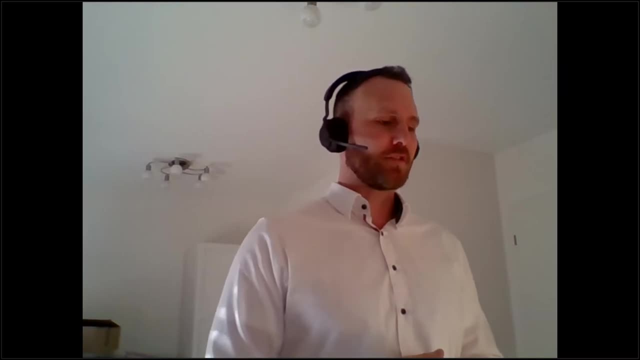 Hello everybody, welcome. It's a pleasure to meet you here for this conference, and a big thank as well to IxSensor Movella, who is organizing and contacting this conference. This gives me the possibility to talk with you about sensor fusion for navigation and. 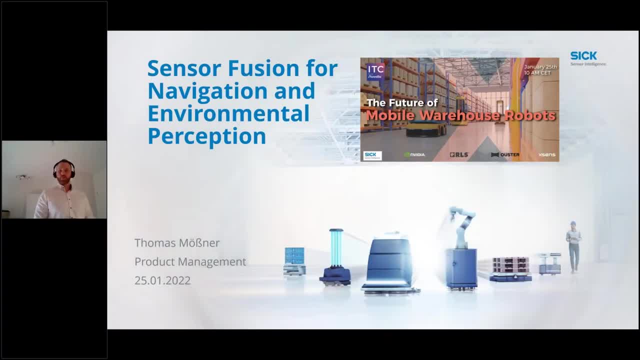 environmental perception. Welcome again. My name is Thomas. I am the product manager for LiDAR localization software at SICK and I want to talk with you and discuss with you a bit. our solutions were for navigation and environmental perception and bringing sensor information together to one point, fuse them to have really higher level functions on top of that. 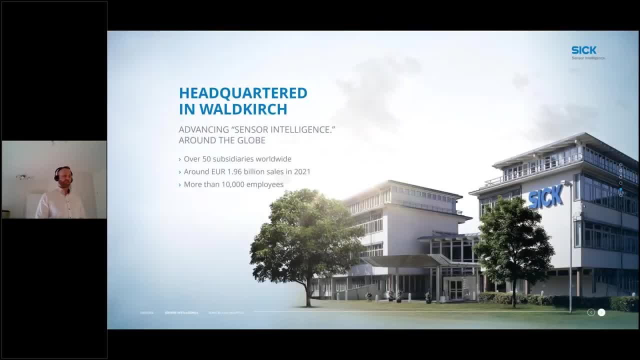 but first of all some few words about sick. he, the company i i working in so um sick, is headquartered in waldkirch. we are best known for building industrial sensors for all kinds of tasks and applications, especially in the fields of factory automation, logistics, automation and process. 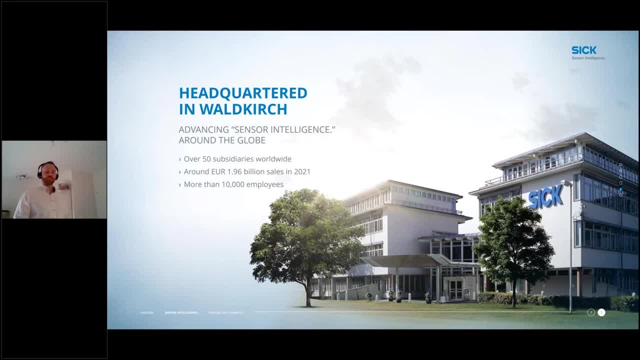 automation. we are a global company with over 50 subsidiaries worldwide, so you contacted us wherever you're located at on the world. um, we made roughly 2 billion euros in sales, yeah, last year, and we did this with more than 10 000 employees spread it all over the world. 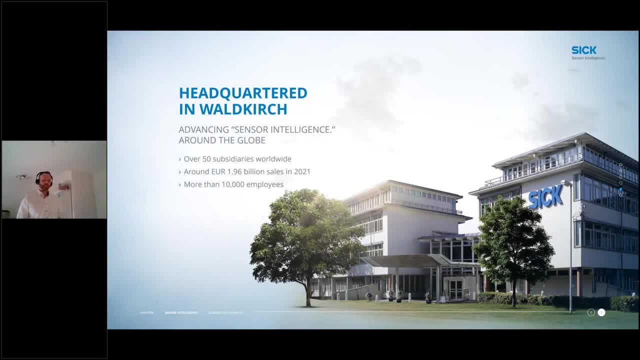 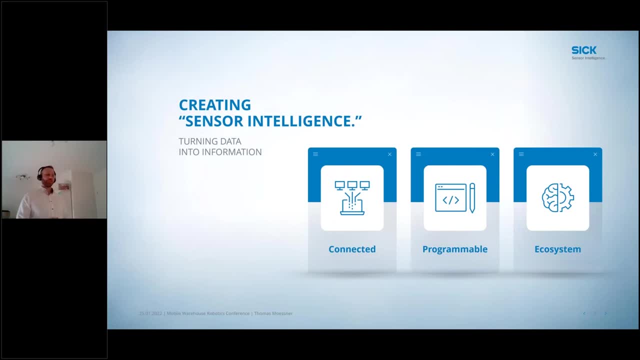 the claim of sick over over several years. right now is creating sensor intelligence. so our major goal is not only building up um high quality industrial sensors for all kind of applications in the fields i mentioned as well, as we want to put some intelligence into the sensors itself, but as well. 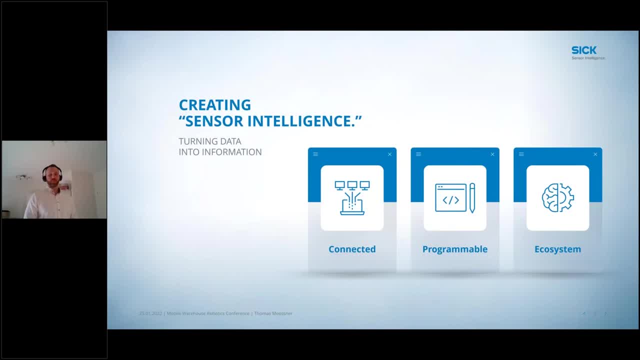 we want to put intelligence into the typical applications we are seeing at our customers. so the idea behind is basically not only providing the measurement data with with our industrial sensors. we really want to turn the data into information, to give you a chance, or to give us the chance, to give you a real solution output which really 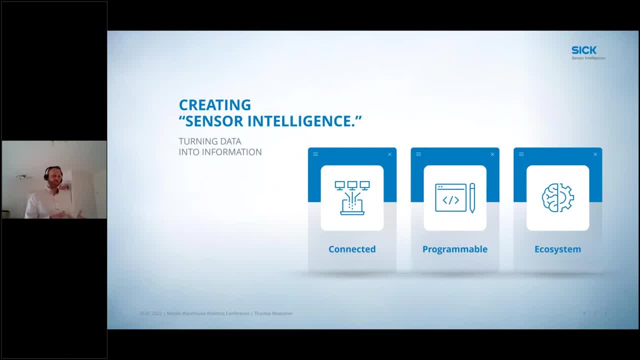 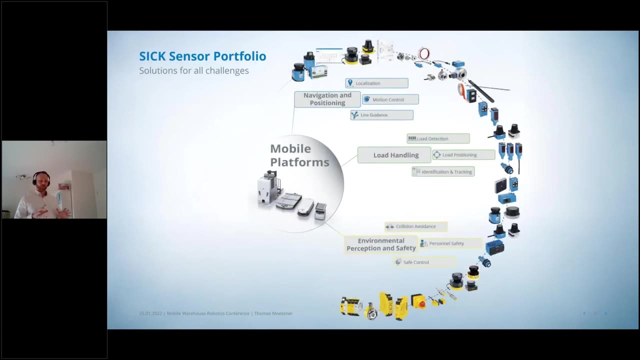 solves directly the application itself. We want to do it in a connected way and in an open manner, so thinking always a bit in a kind of ecosystem. Today I really do not want to point out all the different sensor solutions from SICK. 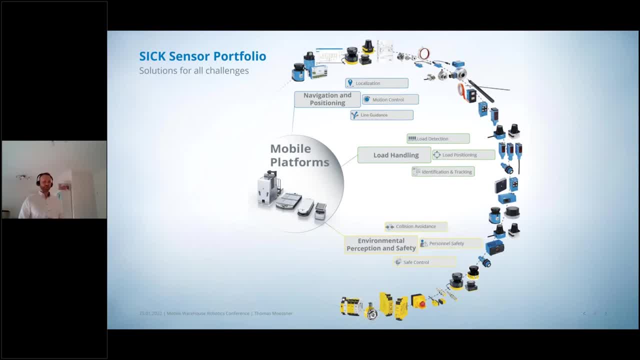 but allow me just this brief slide to highlight what broad sensor portfolio SICK has to attack or to tackle all the typical challenges we are seeing in the mobile robots or mobile platforms market. So we can state we have solutions for all challenges. Maybe SICK is best known for its safety solutions. 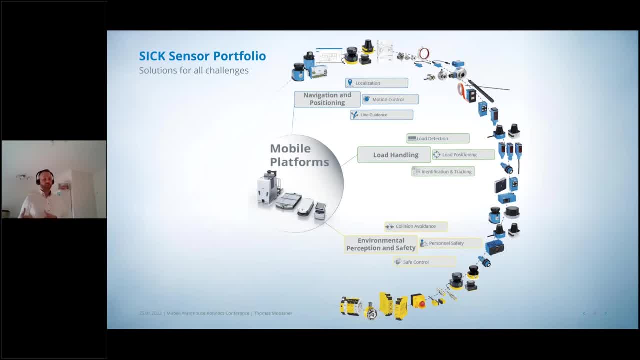 and environmental perception, generally 2D LiDARs, but as well 3D LiDARs. We are focusing as well on the SICK, on typical load handling, task and navigation and positioning as well. So there is a broad portfolio we are having. 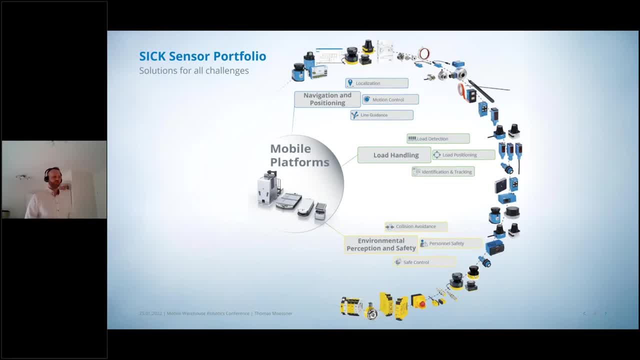 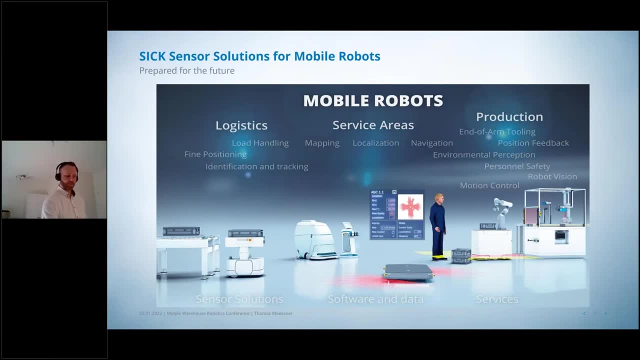 but the focus for today, or the focus for me and my presentation for today is really looking on specific typical applications on mobile robots and for taking more the focus on software and data itself, And I brought with me some or two simple examples for where we are already fusing the data which 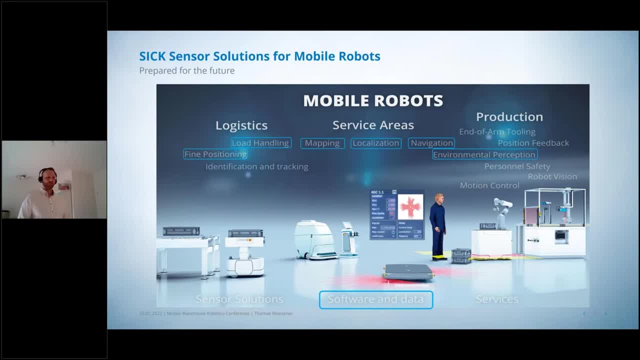 is available from different sensors to a higher level information, And I want to do that with this application. examples for localization, mapping and navigation, but as well one example for environmental perception, for a load handling and fine positioning task. So, starting with the localization, SICK already has a long experience in history. 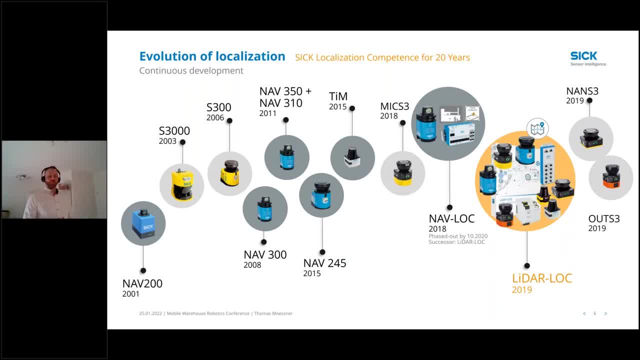 By building up 2D LiDARs especially for localization tasks, and then we developed continuously towards reflector localization up to a solution which is now working on contour, so a contour-based localization solution. But we always want to improve our offerings. 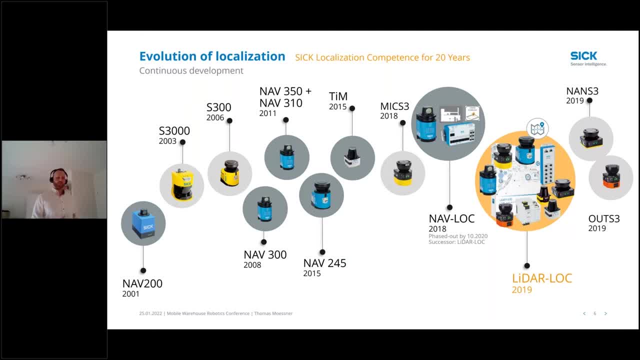 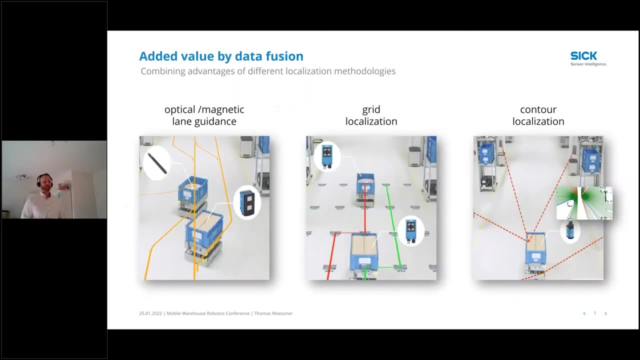 towards additional functions and, as well, implementing additional sensors as well into our solutions, to be always prepared for all the challenges and the tasks which come up in the mobile platform market. And if we just take this localization examples itself, there are basically three typical solutions which are spread out there in the market. 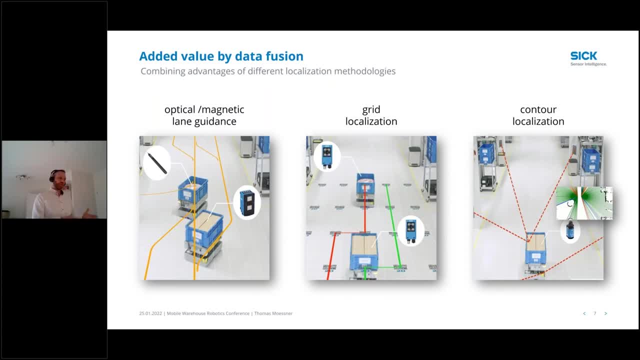 They are all coming with their own advantages. For example, line guided systems. they are mainly easily to implement on the vehicle itself, but as well to deploy this out there in the fleet or on site, as well as the grid localization solution. 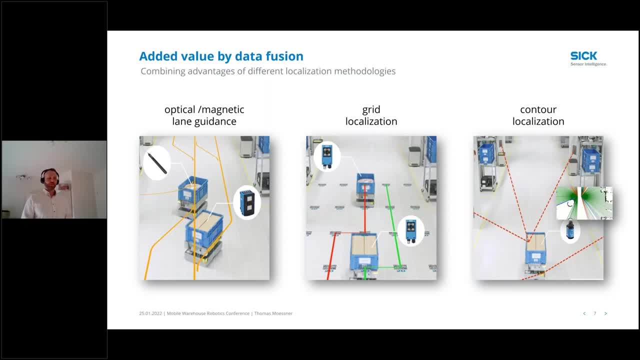 which is just using a simple grid on the floor to localize up to contour localization, which is maybe the most flexible one to use where contour data is taken into account, And this contour localization solution itself is maybe in some ways a bit more, needs a bit more expert knowledge at it. 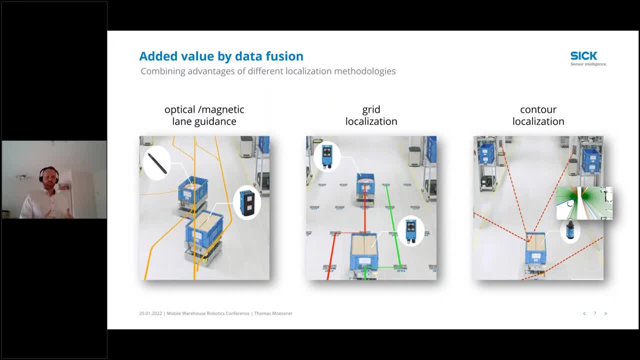 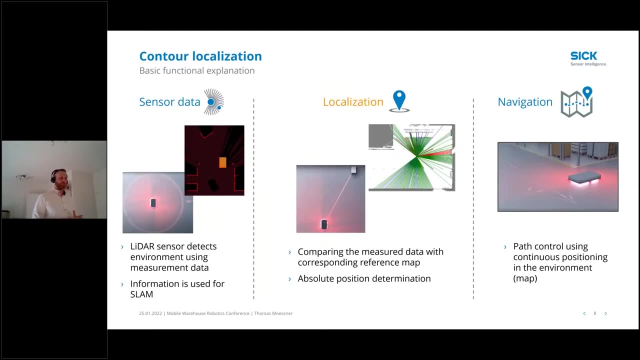 So, again, why not combining different technologies, fuse them together to really have a more easy to implement or, as well, a higher robustness of the solution itself? And this is my as well, my example for today. But first of all, I want to have a short look. 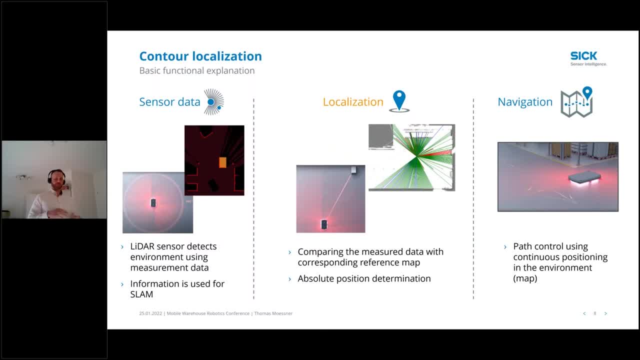 on the basic functional principle of LiDAR localization, so that we are all on the same level. what I want to talk about. So, basically, we are taking the sensor data coming out of a LiDAR sensor which is detecting the environment. 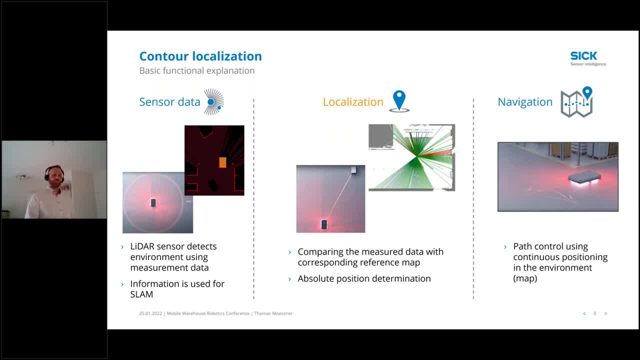 This information is used for creating a kind of reference map. Then in the second step, during the localization task, we are comparing this measurement data coming from the LiDAR sensors with the reference map, And the software, in this case, is able to calculate the absolute position. 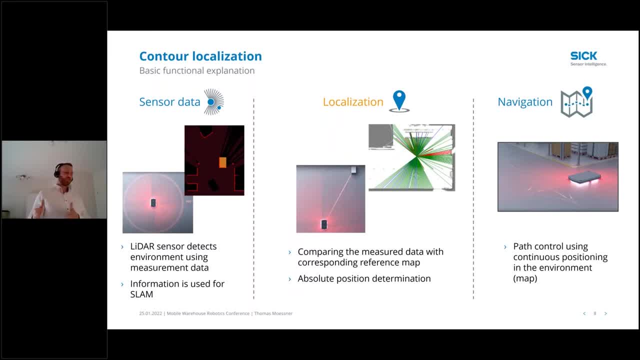 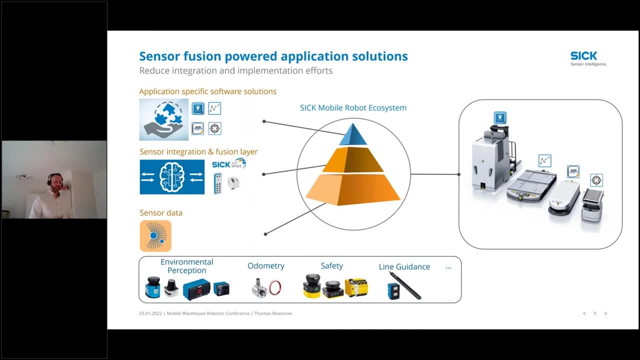 and output this to the second or third point, to for navigation or path control functionality of the vehicles. So this for the basics. And now why, when we are thinking of fusing this information control, localization could be seen as a base sometimes. 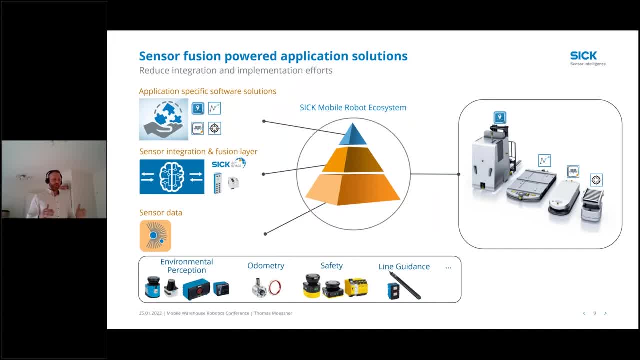 but in general, the approaches or the idea is really to look on the systems on the market and how they are equipped with, And what we can see is that a lot of sensors are already on the vehicles itself, like we've seen in the previous presentation already. 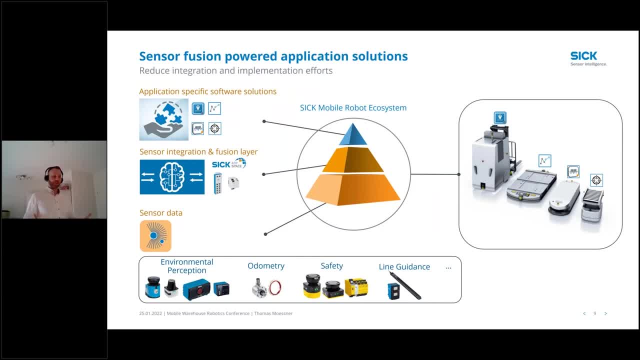 And we can use this existing information and data already and bring them together in one, let's say, integration and fusion layer, And SICK really want to as well help our customers and you to bring this information together in a simple and easy way to do the synchronization. 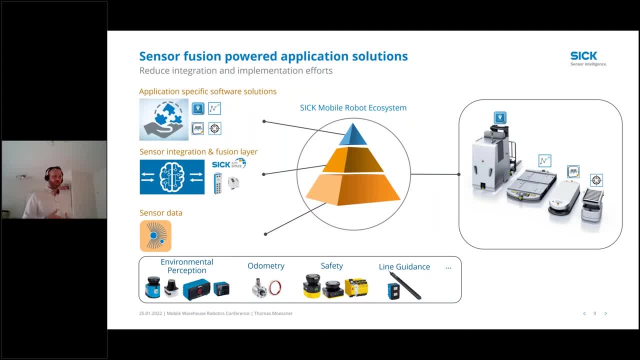 and to bring the data together in a to a point where we can then build higher level functions on it by application specific software solutions, For example. an easy example would be: control localization based on LiDAR sensors is already fusing this information with the data coming from the encoders. 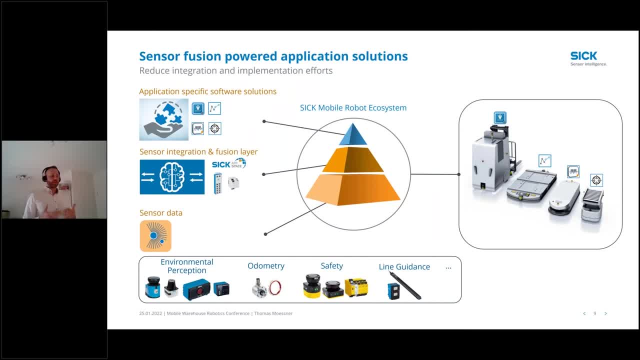 So, speaking about encoders, motor feedback systems in terms of odometry, but as well, there are a lot of systems out there in the market which are still, you know, being designed, guided or using a grid localization, or maybe having additional sensors like ID readers. 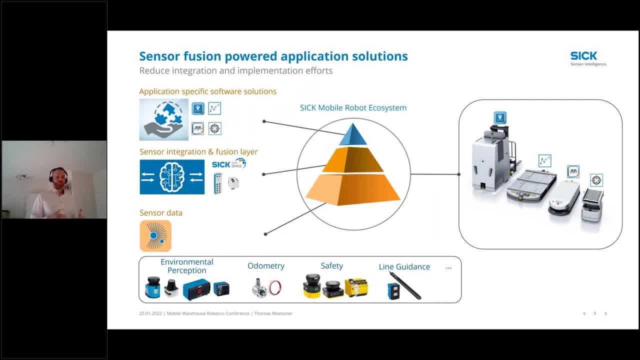 already equipped And we can use this information to just bring all the things together and make things more robust or maybe easier to implement. So this is the basic principle And to maybe bring it more to a concrete examples I brought to with me, The one is: 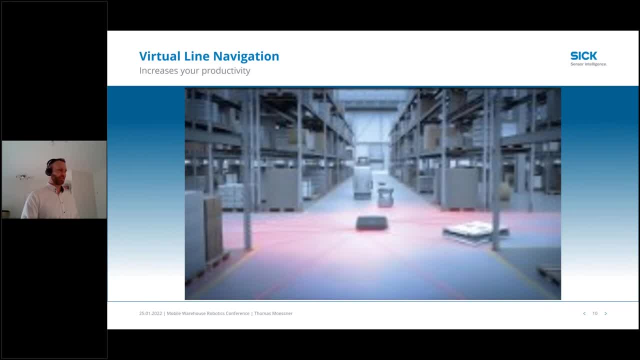 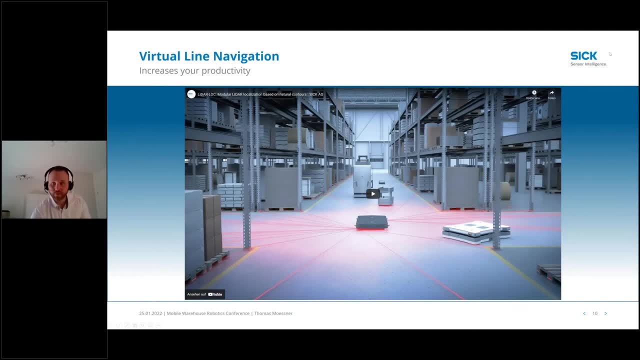 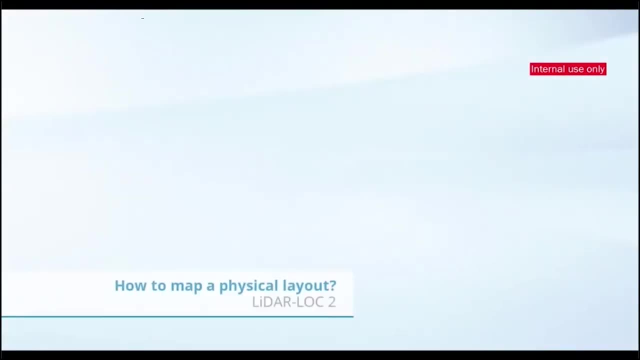 the virtual line navigation, like we call it, this kind of feature extension package where we see a possibility to increase your productivity. And now I need to just switch over to the video, just a second. So in this case, in the first example, we wanted to focus on line guided systems. 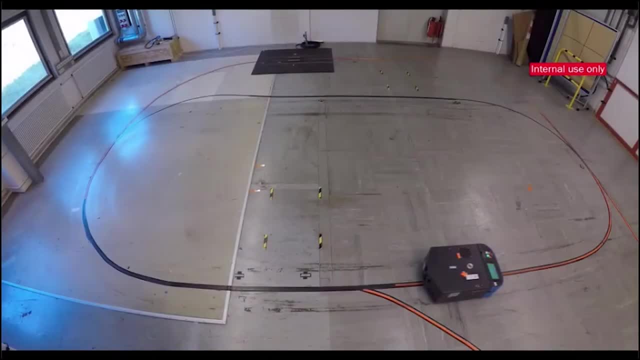 So, when still there are a lot of out there systems which are equipped with a line guidance sensor or a grid localization sensor And for anti-collision, but mainly for safety reasons, they are as well equipped with a 2D LiDAR sensor. 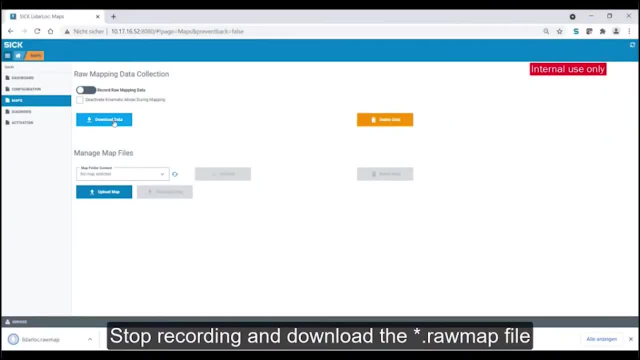 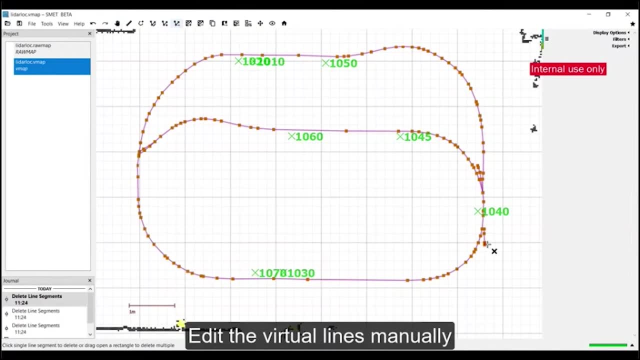 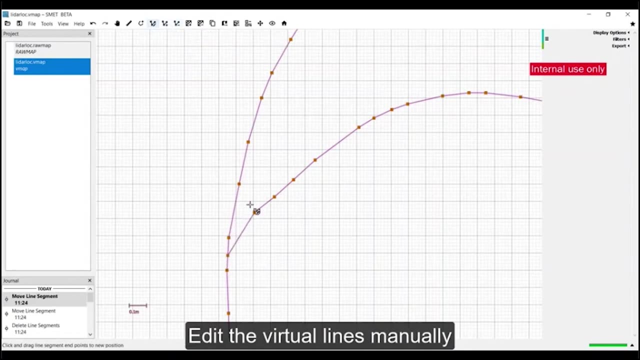 So we developed a software solution which is able, then, to record all the information which is available, So not only the contour information, as well record the physical lines and texts on the floor, And this is part of the map, then, which will allow the software to output a kind of 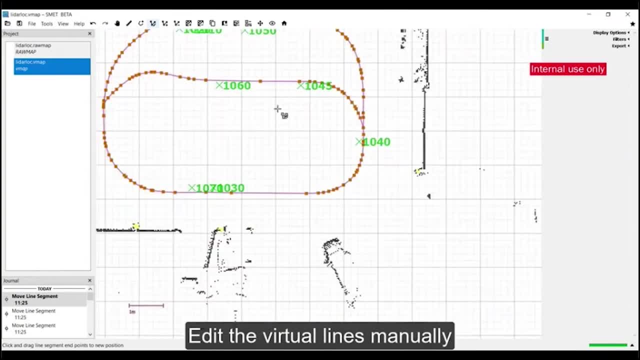 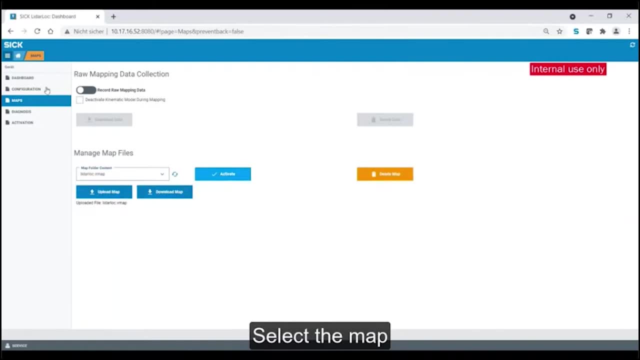 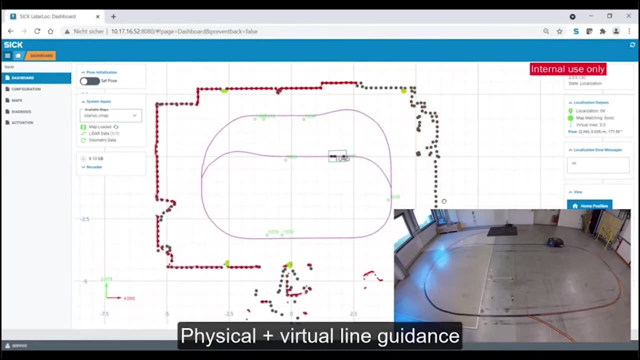 virtual line signal, And with this virtual line signal we have, then, three major possibilities how we can use it. First of all, increase the productivity of existing systems. So the typical pain point for line guided systems is because of we are in tier of the lines. 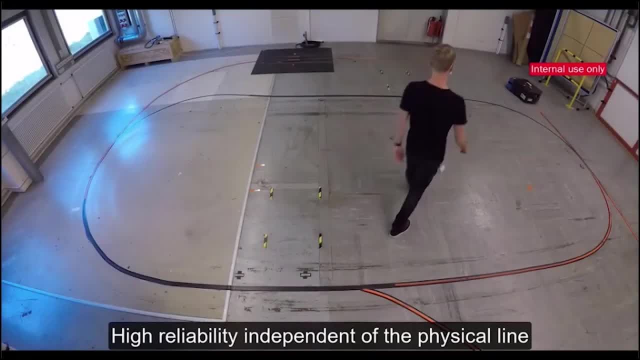 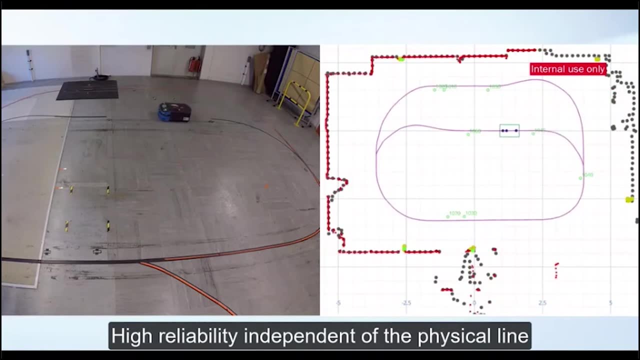 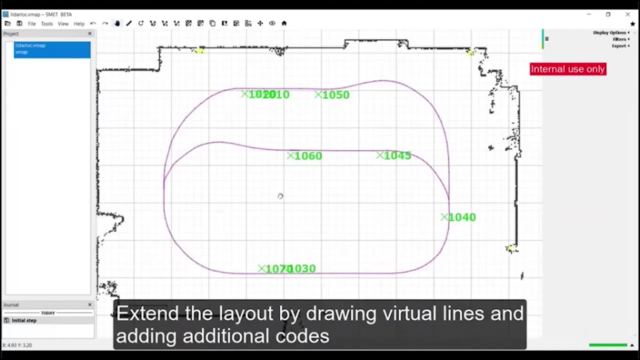 and they get damaged And sometimes this will decrease the productivity dramatically And the software allows them, or the software which is built on top will allow to output a virtual line signal which acts like like a real physical sensor. So it's just a second output with a relative pulse information. 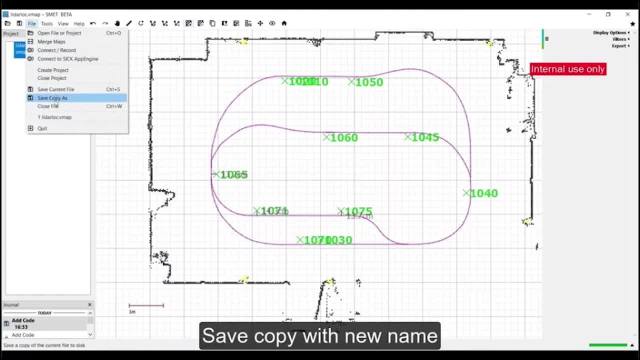 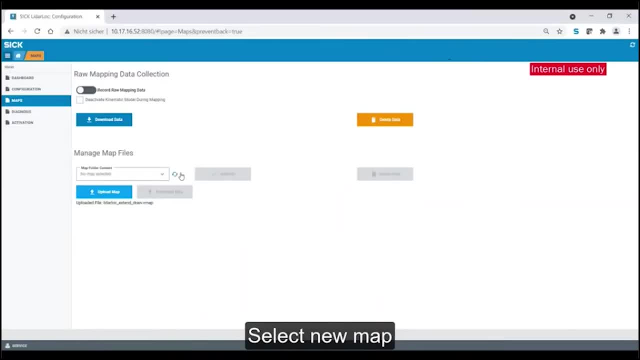 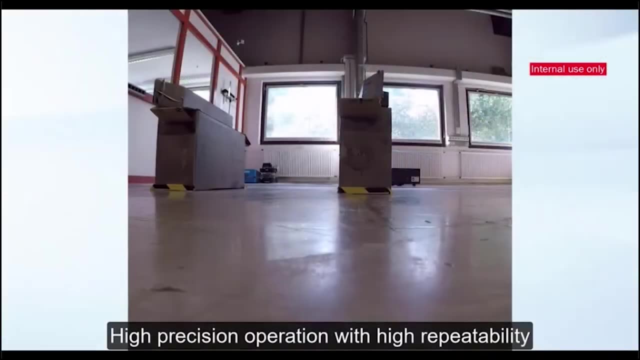 which then allows the vehicles to just drive over any kind of defects in the line. A second possibility which then came up when developing this kind of system is that during the mapping procedure and using our mapping tool, you're as well able to draw some lines. 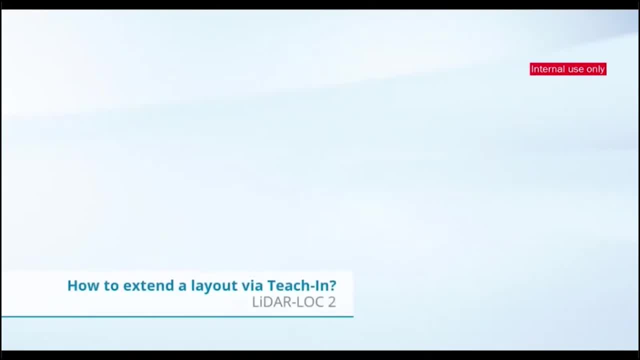 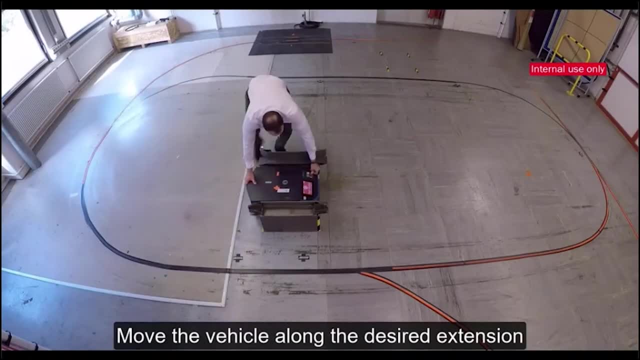 So you do not need to do it physically on the floor. So with this step of virtualization of the real environment, you're as well. it as well allows you to plan and simulate some or test some things virtually as well, by drawing lines. 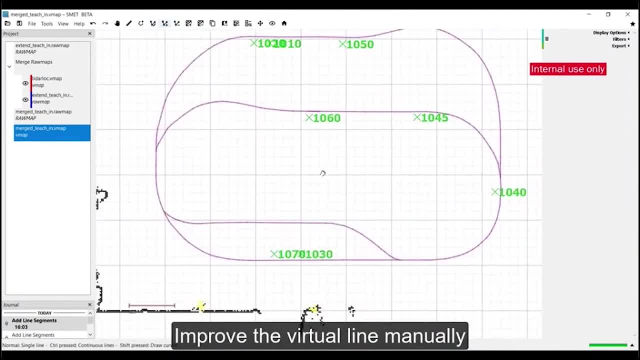 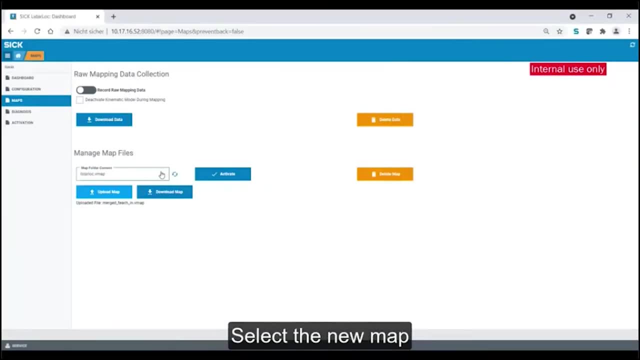 or in this case, you as well, can teach in some, some passes, So by moving the vehicle manually with a joystick or just by hand, so the line or the path can be teached in manually and then it's part of the map. 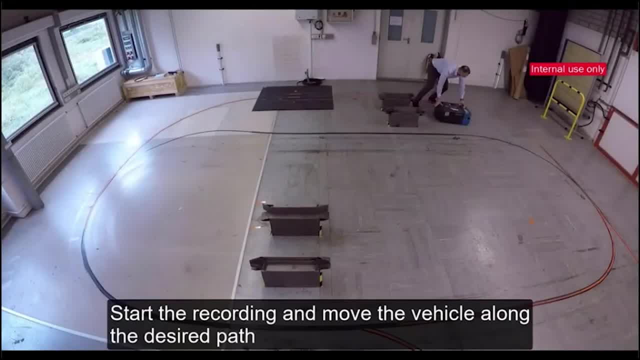 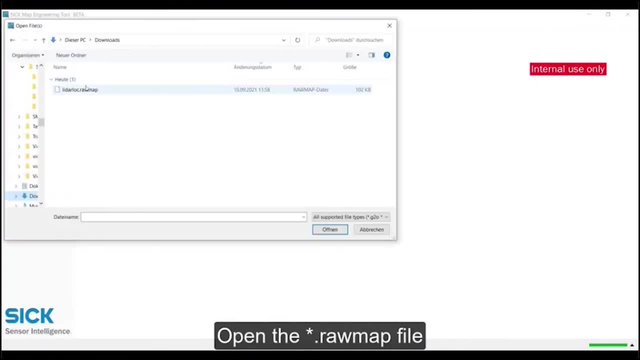 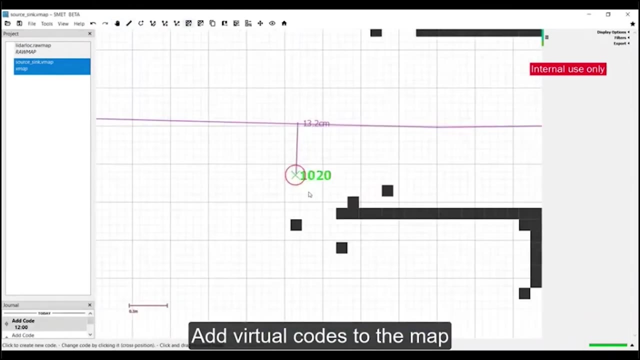 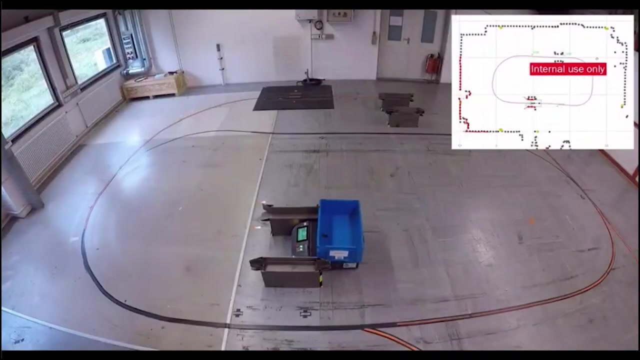 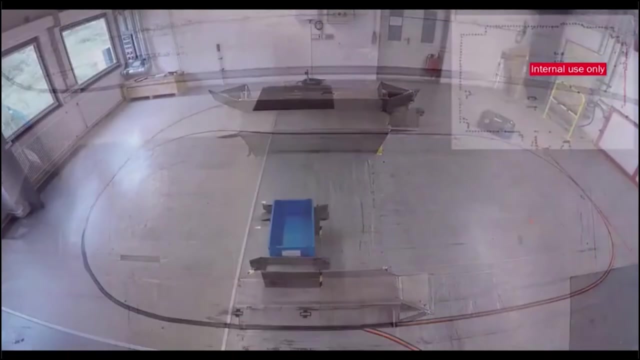 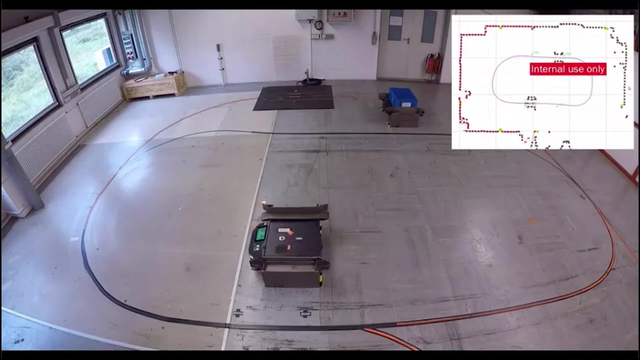 And the vehicle can follow this path with all the two line signals, So you can see what the path is looking like And you can also see the line that you're talking about. So this is a very simple example of how you can do that. 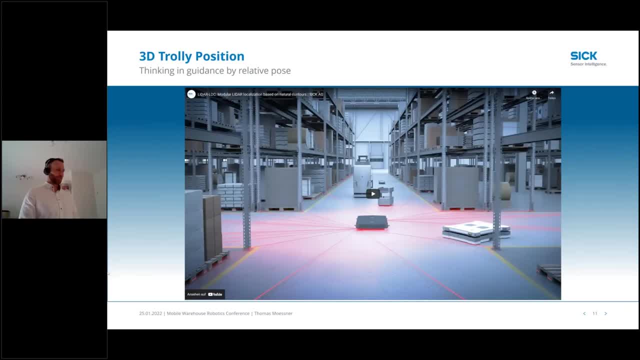 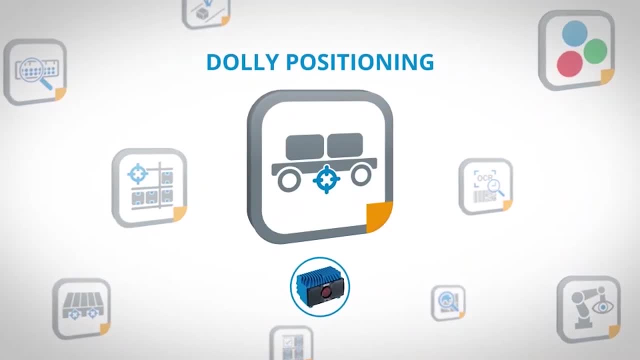 Second example should be shown with the video as well. The idea is to have a typical load handling application, So where the vehicle wants to pick up a trolley, so the trolley is only one example And we are using the in this case. 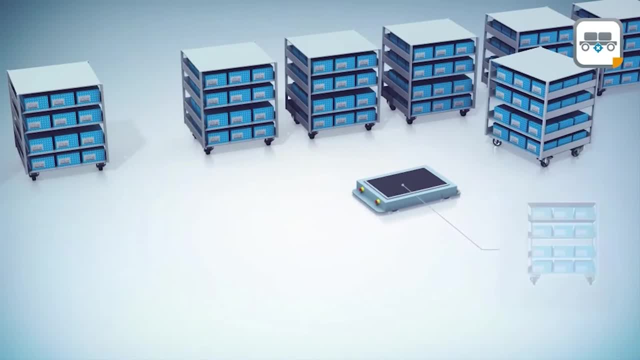 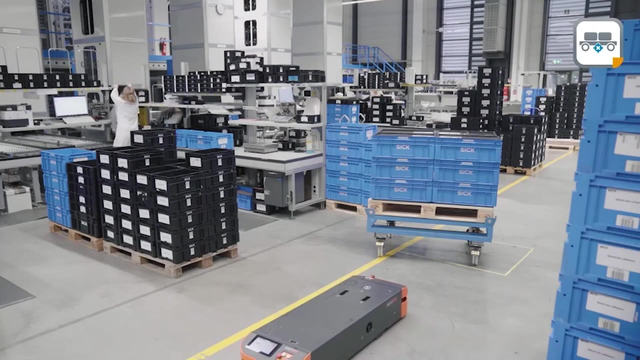 case the 2D LiDAR information coming from the equipped 2D LiDAR and an additional 3D LiDAR which is equipped on the vehicle itself, and this allows the vehicle to have a better environmental perception, not only the 2D layer as well in the 3D layer, and we are fusing these two informations. 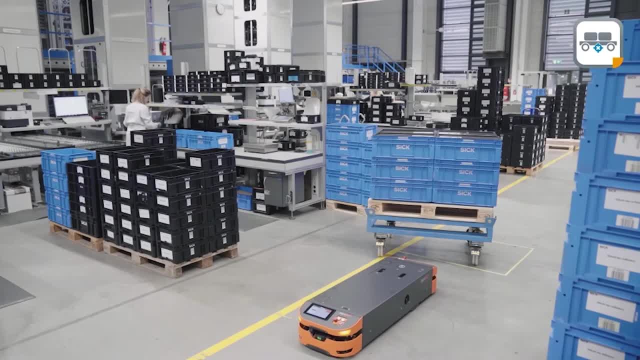 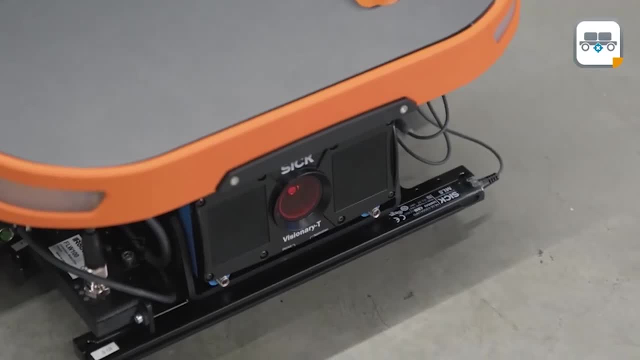 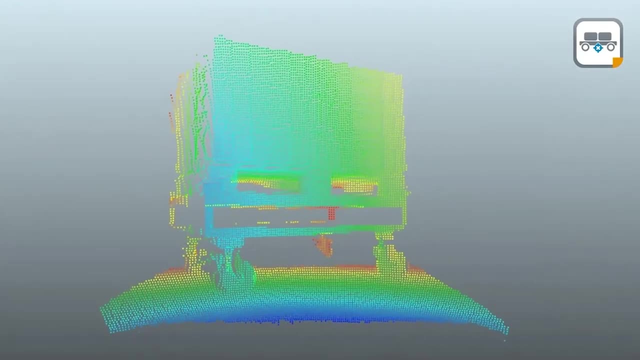 together and mainly due to the fact that we want to detect this trolley, or different types of this trolley, very reliably and robust, and in the video it would have been possible to show you that even if someone is moving in the field, so a human or something else is moving in the field of view. 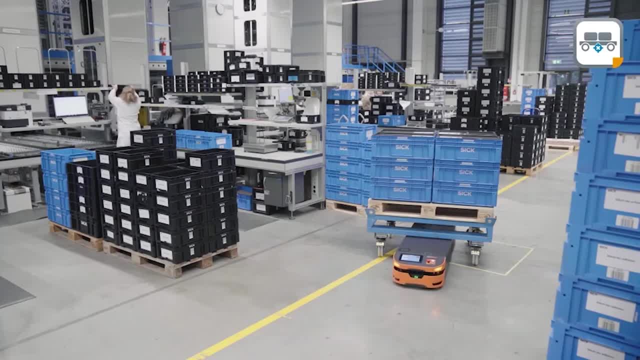 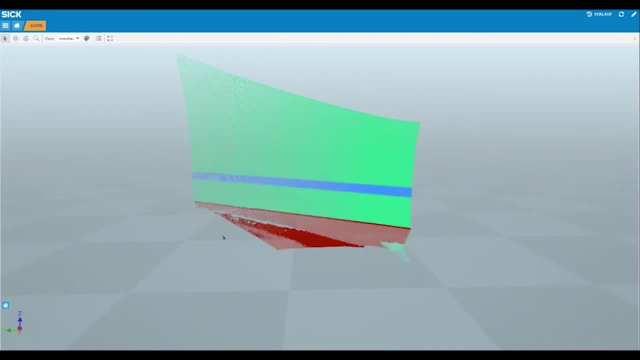 of the 3D LiDAR sensor, we are still able to detect the trolley really robust and reliable, and this is due to that. we are fusing the two, the two datas which are coming on the one hand side from a 2D LiDAR and the second source will be the 3D LiDAR. 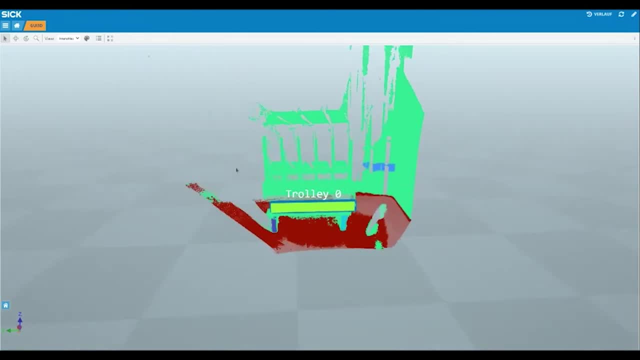 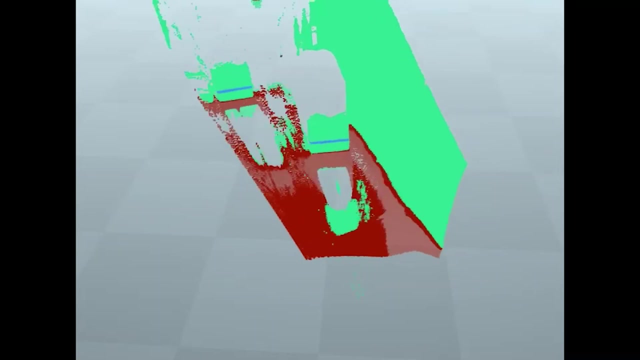 And, as well, a crucial point when when you want to then position relative to to this trolley would be that maybe at some point, or depending on how the the 3D LiDAR device is equipped on the vehicle, maybe the trolley moves out of the field of view of the 3D LiDAR and we will be still able to track. 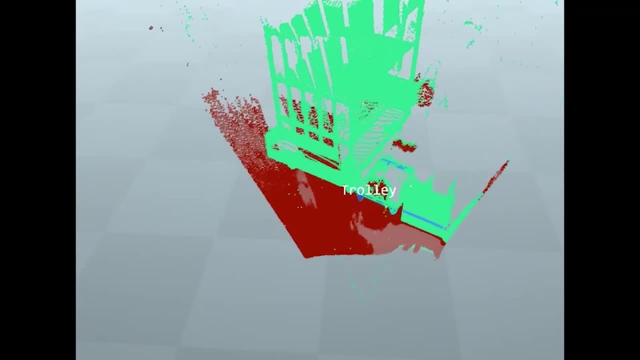 the trolley, even though not the full trolley, is visible in the field of view of the 3D LiDAR, and this is the big, major improvement. By the way, if you have any questions about the 3D LiDAR, please feel free to ask them in the 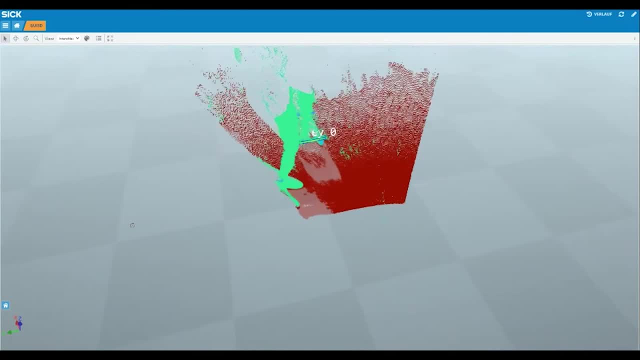 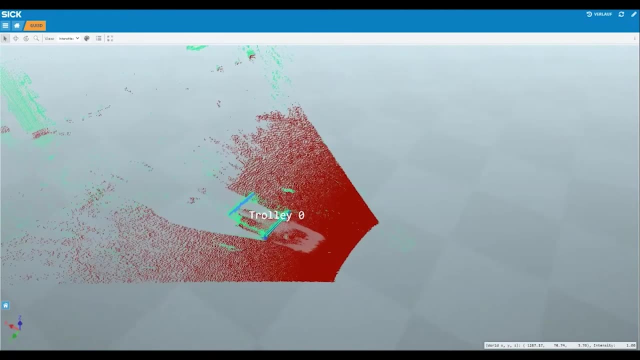 Q&A section of the Q&A box. using this, the different informations together coming from the 2D LiDAR, in this case in the 3D LiDAR, so that we have a more reliable detection at the first point and, as well, being able to track. 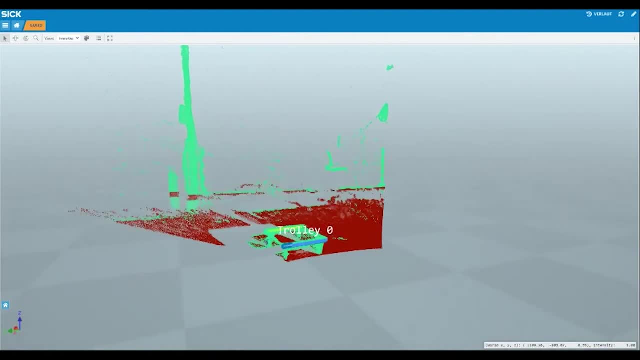 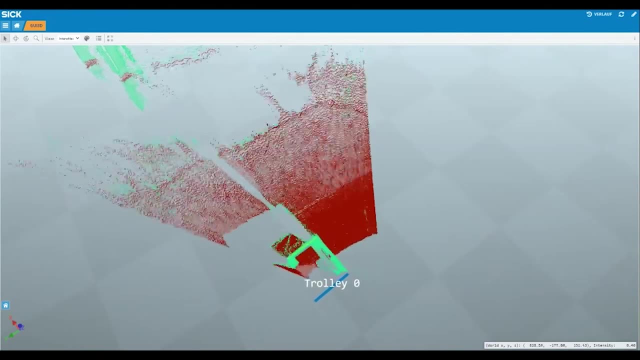 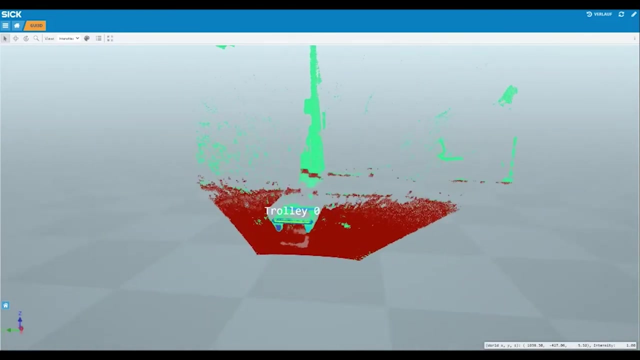 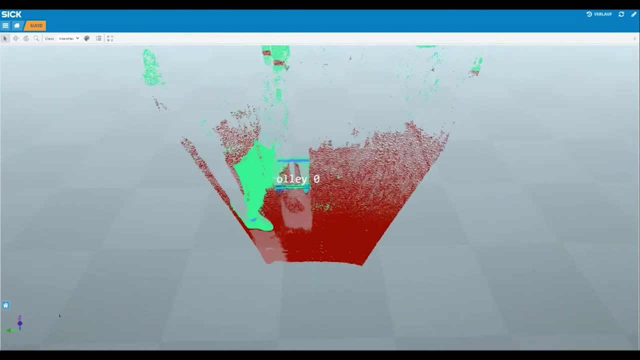 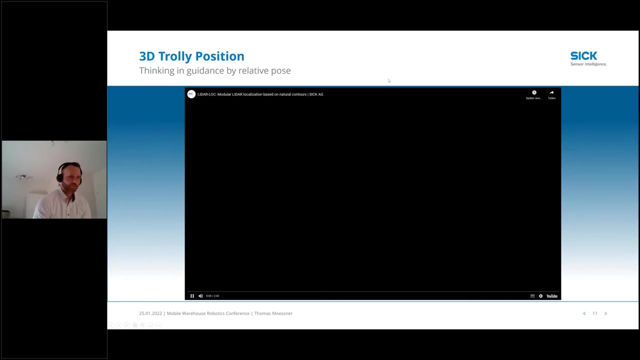 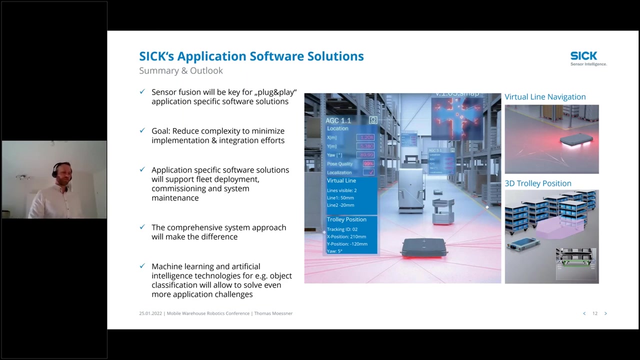 the trolley during movement to really allow the vehicle to position quite precisely below, below the trolley in this case. And in this case I come already to to my summary and outlook. So, with six sensors, specific application software solutions, we are focusing on the most common application challenge. 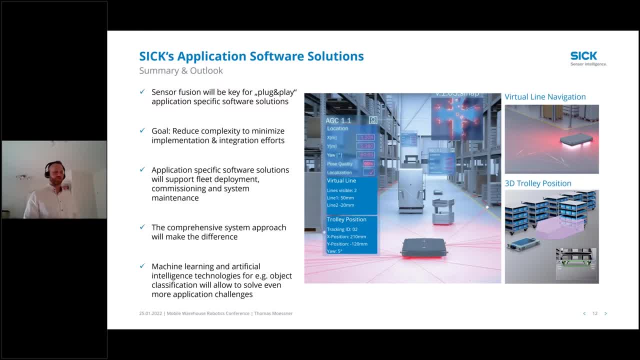 So we are focusing on the most common application challenge, challenges we are seeing for our customers or with our customers, And without equipping additional, without equipping this vehicles with additional sensors or it is not mandatory needed, we take all the information which is already. 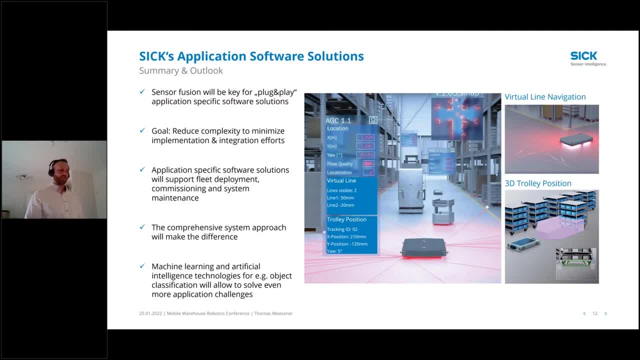 available on the vehicle itself by the sensors used already by the vehicle, bringing it in a kind of integration and fusion layer and build some application specific software on it, And we think, or I believe, that this will be the key for plug and play application specific software solutions. 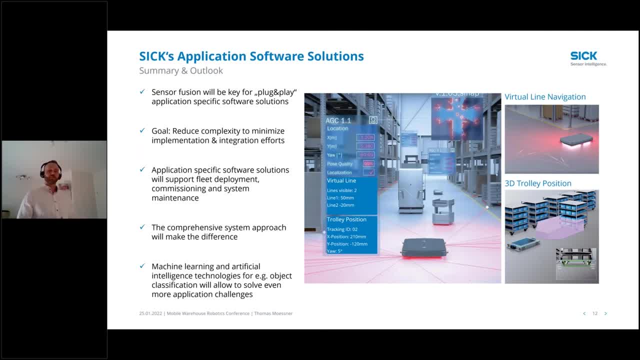 So the overall goal would be to reduce the complexity for our customers or, in general, to minimize the implementation and integration efforts, And this application specific software solutions will support free deployment, commissioning and system maintenance, like the videos would have shown, And I personally believe especially. 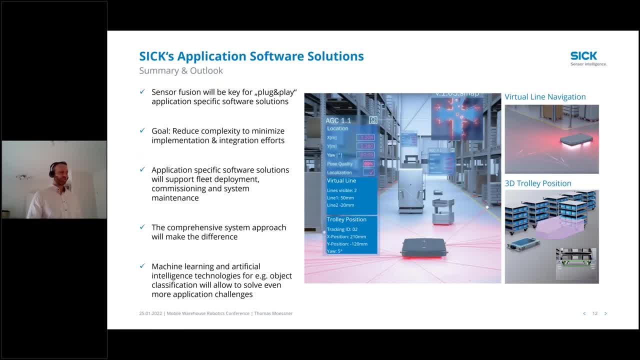 the comprehensive System approach will make the difference. So SICK as well is spending a lot of efforts into machine learning and artificial intelligence technologies. For example, like already mentioned before, object classification tasks, and these advancing technologies and the broad usage of it will allow. 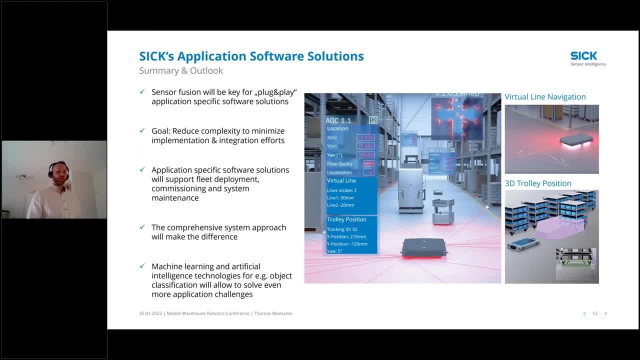 to solve even more challenging applications. But I think in the first step the major point is to really reduce complexity. So using new technologies and new approaches, not to increase complexity. I think the major intention for us all is to reduce complexity. So the implementation in the field. 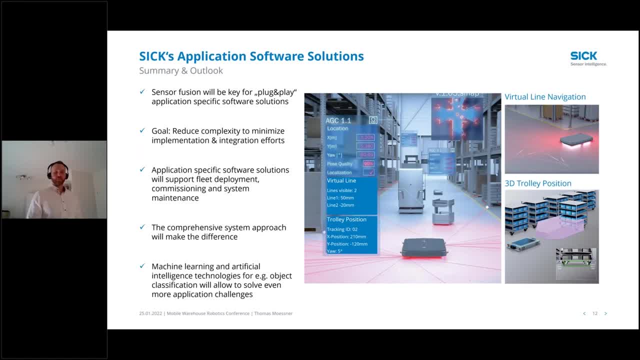 will be as effective and efficient and convenient for everyone, And you won't need only experts out in the field, So a typical trained engineer is able to conduct it And thank you with that. I want to thank you for your attention. Thank you. 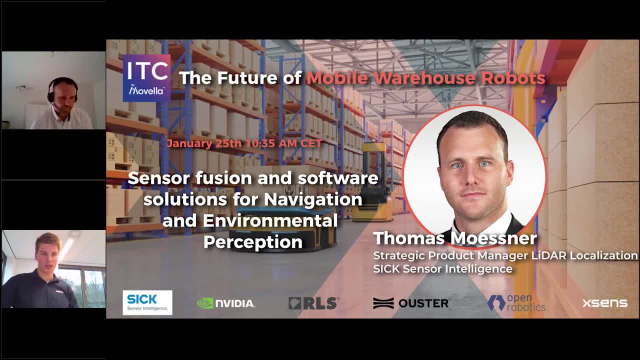 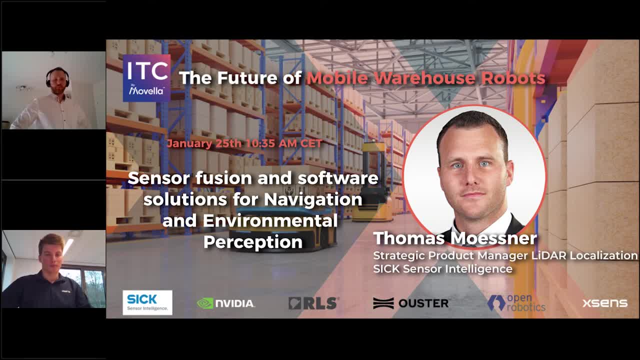 lighters in the US and India. Yeah, I know that the situation maybe is a bit difficult. It's just because of the sourcing situation overall in all industries and the market. I'm personally not the product manager for the safety sensors And I do not really know the exact facts. 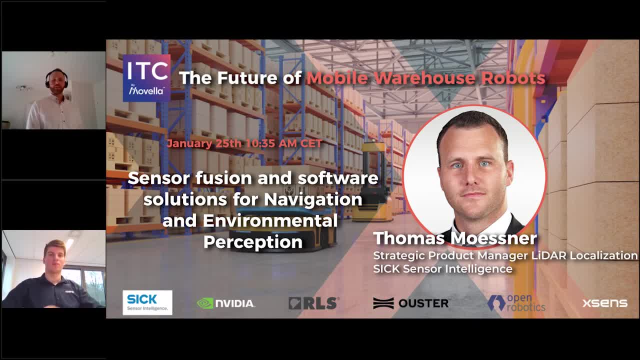 I just know that the situation maybe is a bit complicated, But SICK is working really hard and constantly on improving that And all I know is that no critical situations are occurring right now. But yeah, maybe this needs to be addressed to the right channels to get a really clear and concrete 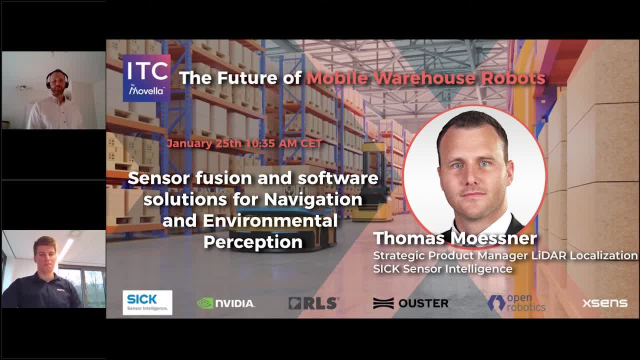 answer. specific answer to this question. OK yeah, we of course share it with you, And then you can hand it over to the right person. Then the question: this software comes with your dedicated hardware, or can we use it as a library on a vehicle's computer? 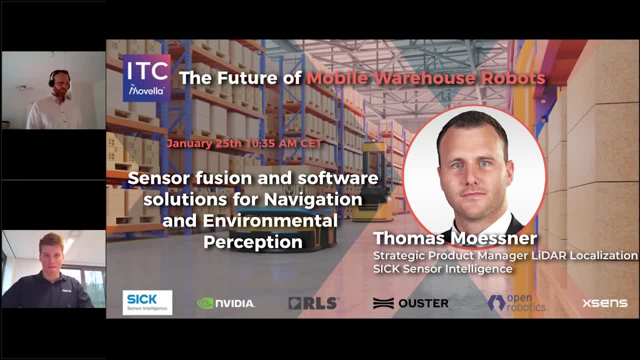 for example, a ROS-based computer. Yeah, you can use it on a typical iPad, PC or vehicle controller, like you already have it or want to use it. We are especially for the controller perspective. we are following an open concept, so that as well. 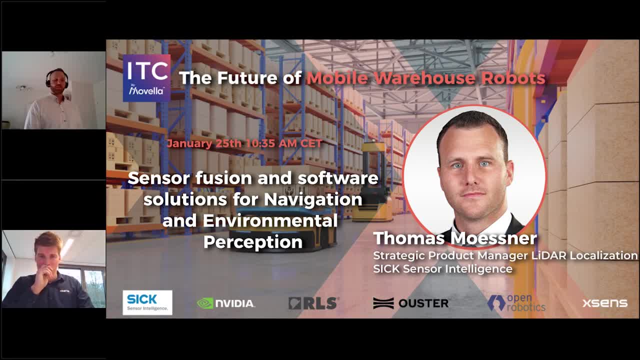 these solutions can be used not only on SICK devices and SICK controllers. In this case, we would allow as well, or we already implemented or developed it in a way that it is possible to use it on the typical IPCs and controllers. 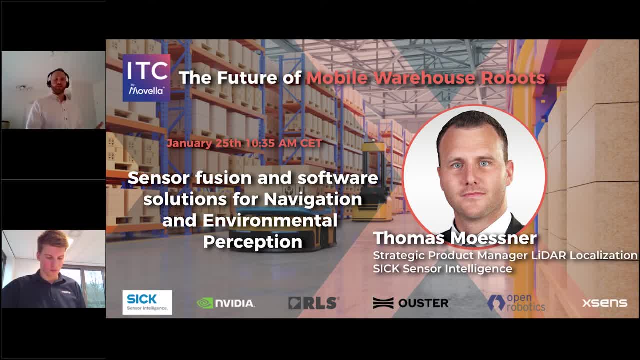 out there. It's just one point to mention. One view on the resource situation is maybe typical or needs to be done, But with all these software solutions we are developing, we are always focusing to do it as resource-effective as possible. yeah. 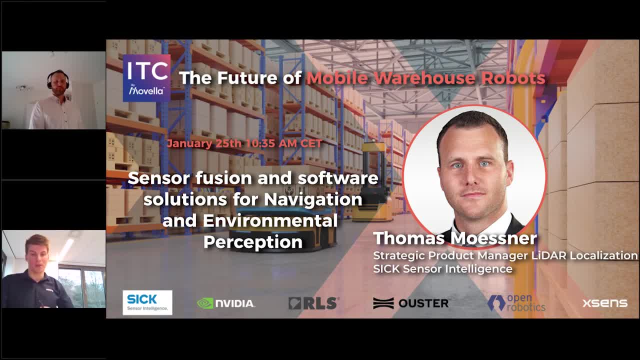 OK, in case. thank you for that. in case of an indoor AGV, the application, the environmental conditions will be different than outdoor. How do you think about this? I agree, And they are really completely different, And outdoors, especially the wide ranges, may be a limit. 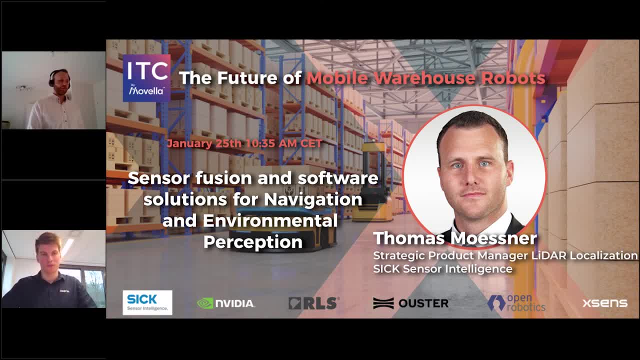 Some typical approaches which are already proven in the indoor environment. We have a big initiative at SICK which is focusing on mobile auto automation as well, taking especially these specialties and requirements into account and feedback it with a typical requirements engineering approach towards our sensor development. 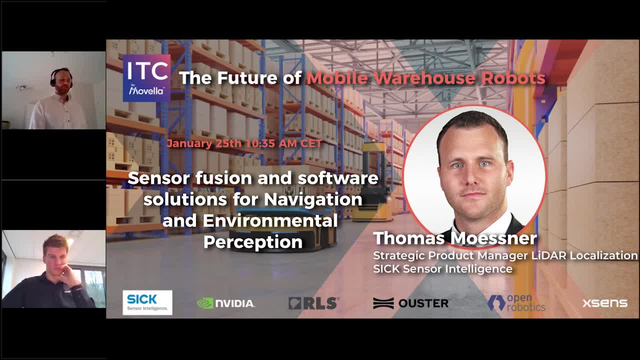 departments, but as well for the software development departments as well. So if there are specific applications out there, we need to have a closer look at it. But generally speaking, we have this as well on our OK, But generally speaking, we have this as well on our. 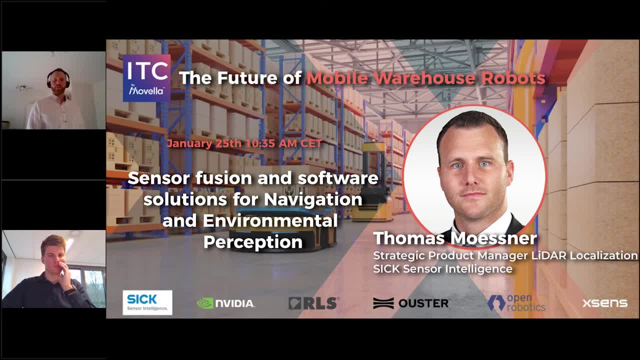 on our radar and some ideas already how to solve it. yeah, OK, now I got thanks for that. I got two questions. I think they're the same. One is: is this software a SICK solution or an open software for other manufacturers as well? 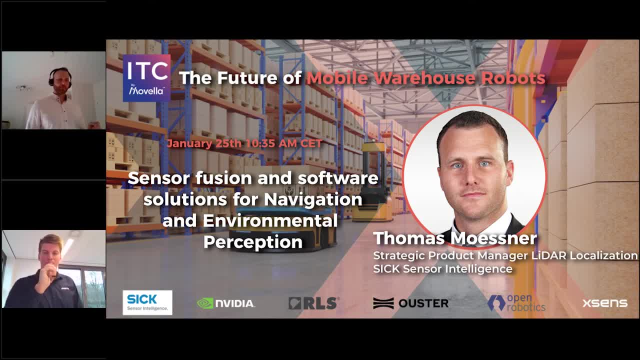 And then: is this software free or not? Yeah, so these two examples I explained only by word. This is a specific SICK software. yeah, And it's based on the SICK app space concept from SICK. So basically, SICK app space is an open concept. 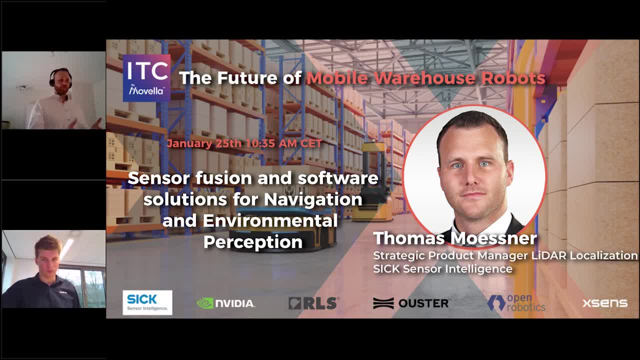 where customers can as well develop their own software solutions in the surrounding, but this need not to be mandatorily done. Our idea is: with this capsuled software solution we want to have a dedicated solution output which already solves one part or some parts of the applications. 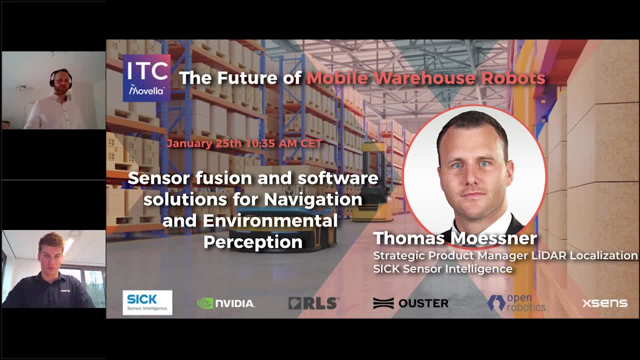 and others can then still stay by our customers and can be done in their typical way, And in this example, maybe with Ross. yeah, OK, and I think it has some. it's close to the one, But does your solution require SICK sensors? 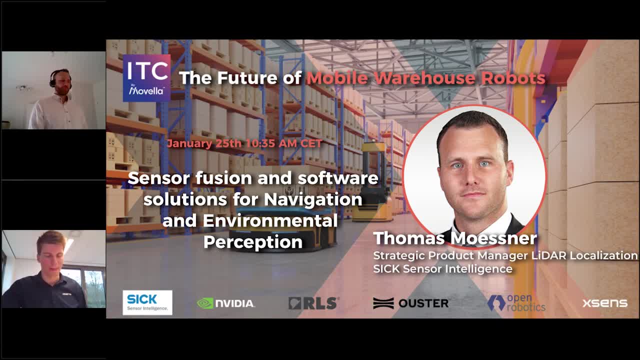 or is it possible to use sensors from other brands as well? Yeah, so generally, as I said, we are following this open concept, especially for controllers. This can directly be seen for these two examples, maybe looking on the virtual line navigation, where we are using physical line sensors. 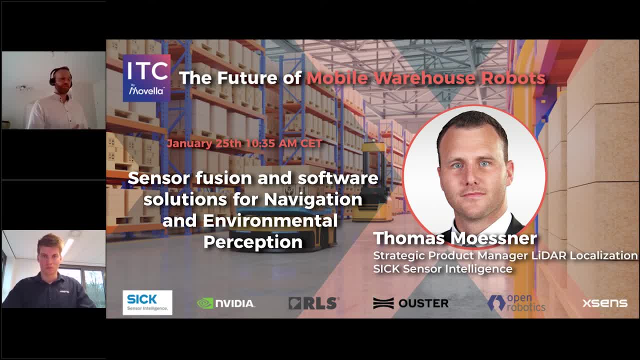 And a lot of systems out there in the market are already equipped with any kind of sensor, And this sensor then can be inputted to our software solution. Where we are a bit more restrictive is by using the LiDAR sensor. This is just because of the contour localization solution. 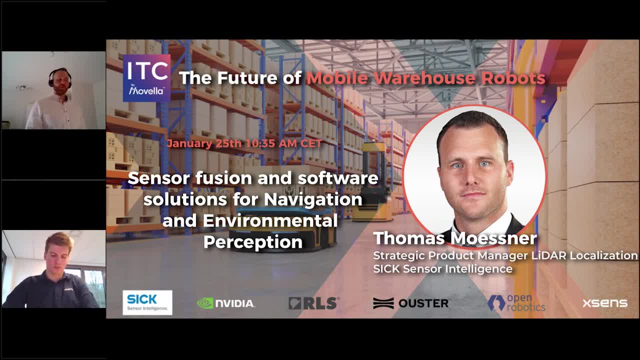 We need a really reliable and good and precise measurement database And there we are, allowing today only SICK, using SICK LiDAR sensors as an input. Yeah, it's depending a bit on how flexible as well we can be in our system approach when always want. 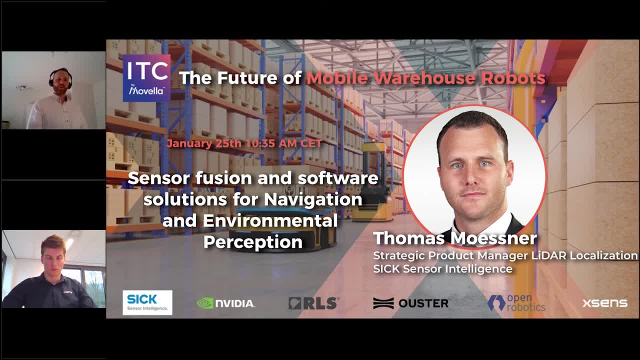 to guarantee the best and most precise and accurate and reliable output? yeah, results to our customers? yeah, That makes sense. Are you considering autonomy functions for mobile robots as well? Yes, we are, So maybe sometimes there is a differentiation between autonomy, so the vehicle itself.